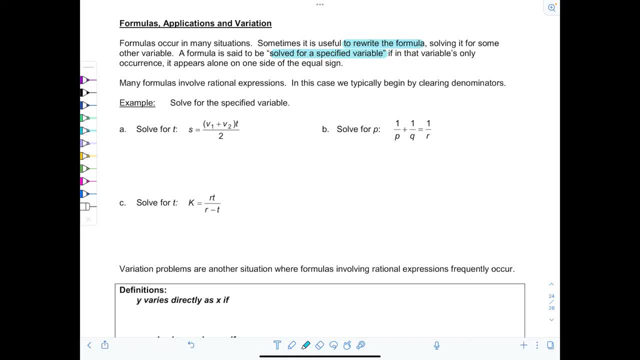 specified variable. Okay, so let's just get some practice here. Example: solve for the specified variable. In example A it's asking us to solve for T or to isolate T. Okay, we'll look over here, on the right-hand side of the equation, where T is, and I'm noticing two main things that are: 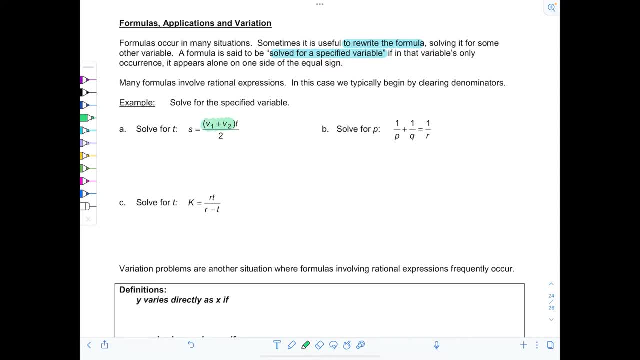 in isolation. There's this V1 plus V2- in parentheses, being multiplied by T, and then also, I notice T is being divided by 2.. So let's go step by step and remove each of those elements right that are on the right-hand side of the equation with T. So, first thing, how about we multiply both sides by 2? 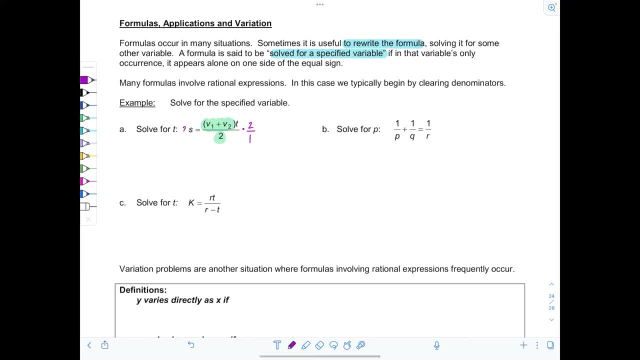 or 2 over 1, right. That way you can cancel out that 2 in the denominator. So now bam bam. on the right-hand side of the equation we have T. So now bam bam on the right-hand side of the. 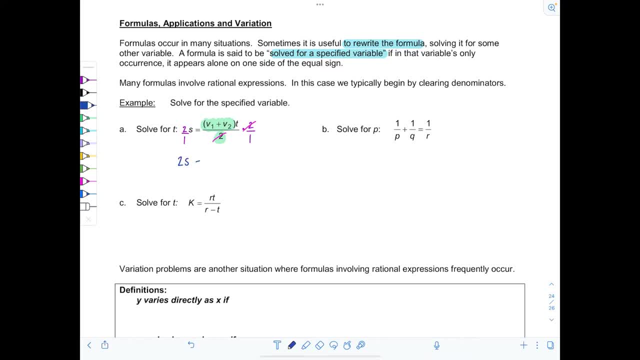 equation, it's gone. On the left we have 2S equals V1, plus V2 times T. All right, good, and don't distribute through on the right-hand side, because, remember, we're trying to get T by itself. So I 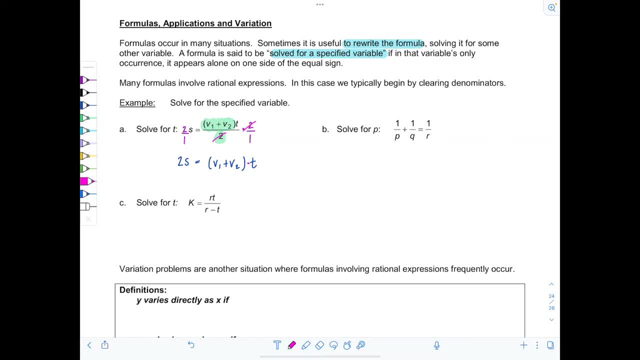 actually want to get rid of V1 plus V2.. Remember that's being multiplied by T. So let's just go ahead now and divide both sides by V1 plus V2. And we're pretty much done. So notice here: V1 plus V2 cancels. on the right-hand side I have T. 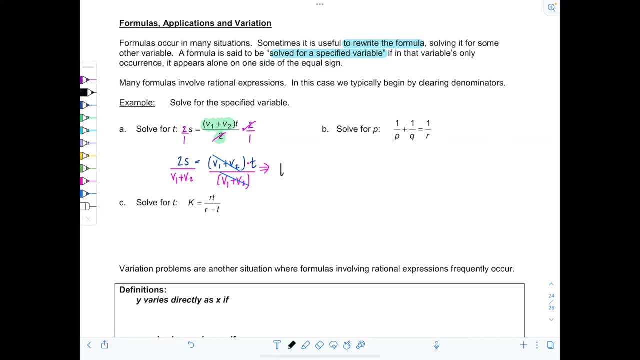 all by itself. I'm going to put T on the left, So T equals 2S divided by V1 plus V2.. And that's it. So let's go ahead and box it. We finished part A. Cool, All right, good. 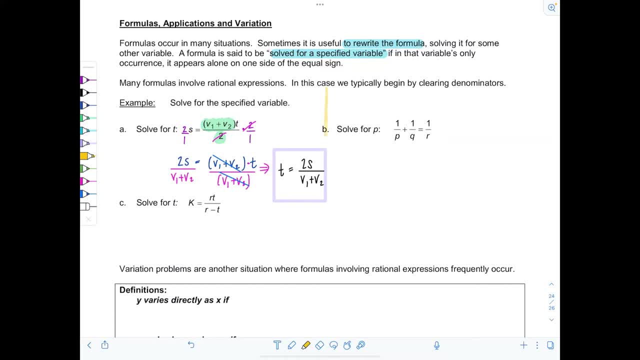 Let's move on to example B. In this case it asks us to solve for P. All right, Well, first thing I noticed this is a rational equation because the variables- more than one variable- appears in the denominator. So think back to when we solved rational equations. If you forgot, I'll link. 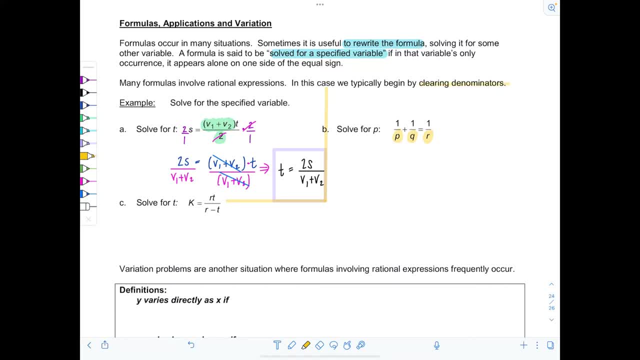 the video right here. The first thing you want to do is clear your denominators, meaning you want to multiply by the LCD of the equation. So the LCD of the equation is going to be the number of PQR and that distributes to each of the terms in the equation. Okay, good. Now this is PQR over 1,. 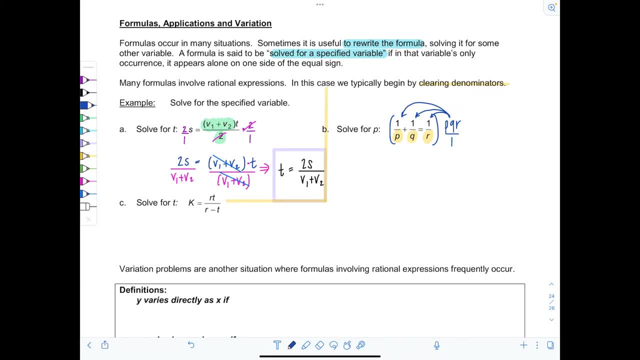 basically. So when I multiply PQR by that first term, by 1 over P, P cancels out. So I'm just left with Q times R plus 1 over Q, The Q will cancel out with PQR, so I'm just left with PR, And then this is going to equal: 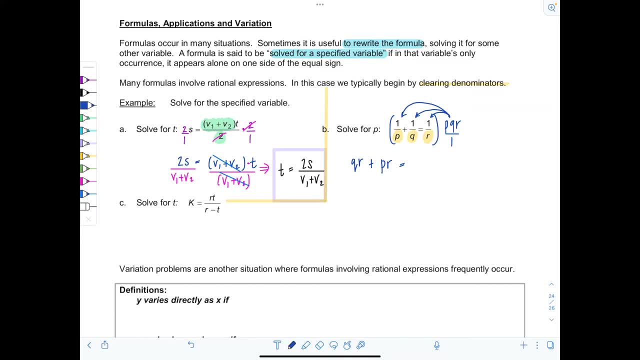 what should I have on the right-hand side? Very good, PQ. Okay, now go back. Always remind yourself, check the directions. Which variable are we being asked to solve for? We're being asked to solve for P, So where is P? P is? I see one here and then I see one more over here. 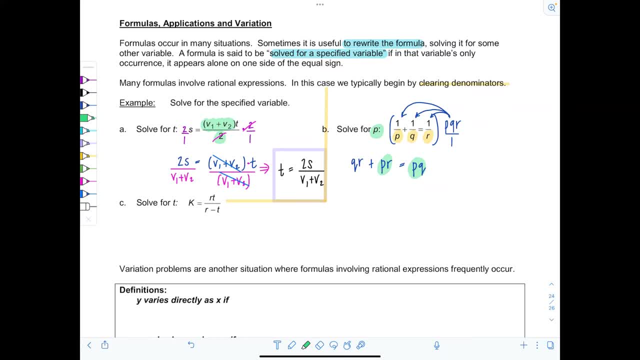 on the other side of the equation. So when that happens, we're going to have to solve for P. So when that happens, the technique is as follows: You want to get all the terms that have P on the same side of the equation first. So let's move PR to join his little buddy PQ on the right. So 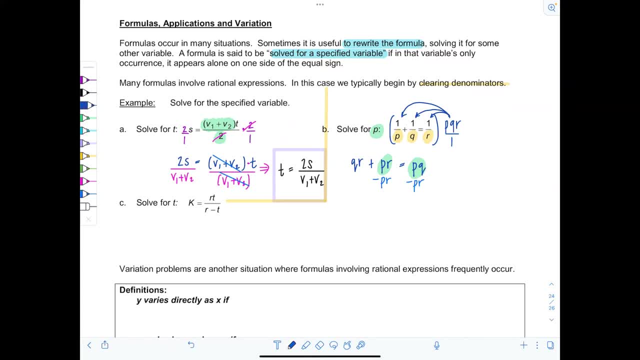 I'll subtract PR And now I have QR equals PQ minus PR, And the reason we do this is now all the terms that have P are on the right. I can factor P out of both terms on the left, and I can do the same thing on the right-hand side And I'm left with Q minus R, And this is all equal to QR. 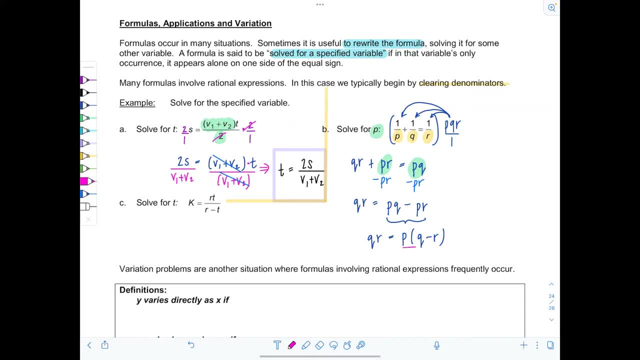 All right, good, And then we're almost done. Remember, we're trying to get P all by itself. I'm going to divide both sides by Q minus R, Divide by Q minus R, And then I can write my final result as: P equals QR over Q minus R. 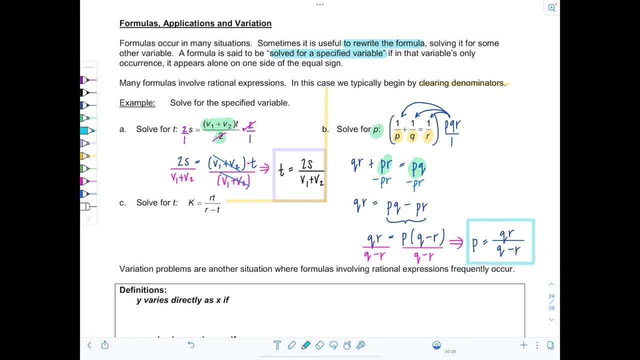 So that process should remind you, if you think back to when we would find the equation for the inverse of a function. same process, Okay, now let's go ahead. look at example C. We're going to solve for T. Ooh, this is going to be a little tricky because notice, there's T up here in the numerator. 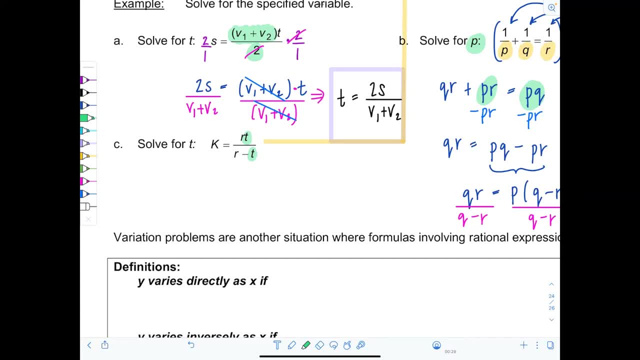 T down here in the denominator. So what we're going to do first, it's a rational equation: let's get rid of the denominator. I'm going to multiply both sides by R minus T, So now we have K times R minus T equals R times T, And then let's go ahead, distribute through. 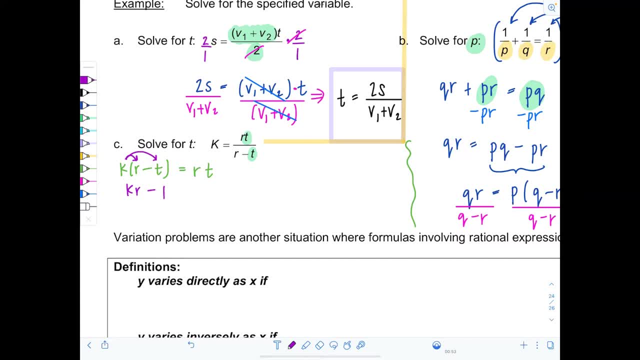 on the left-hand side. So we have KR minus KT equals RT. Good, Remember which variable we're solving for. We're solving for T- I see one over here and one over here- And think back to example B. You want whatever variable. 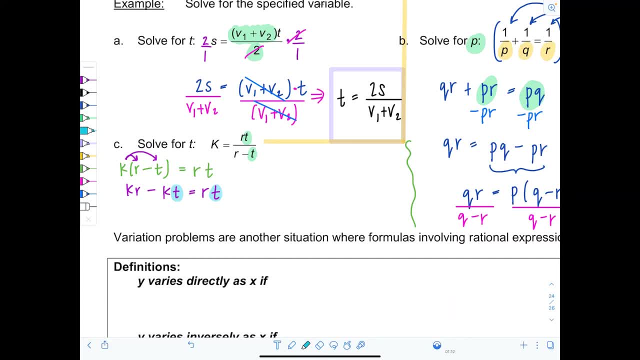 you're solving for for all of the terms that have that variable to be on the same side of the equation, And then all the terms that don't have that variable, the ones that don't have T, have to get exiled to the other side. So I'm going to add KT to both sides. 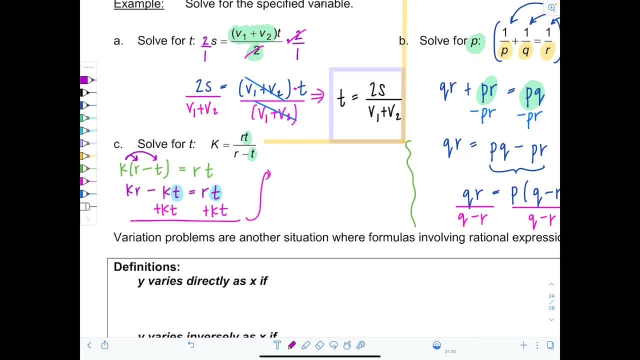 Okay, okay, And then let's see what we're left with here. So now I have: KR is equal to RT plus KT, And then I can go ahead, factor out a T here and I have R plus K. So that's the whole point of grouping all the terms with T on the same side. You want to be? 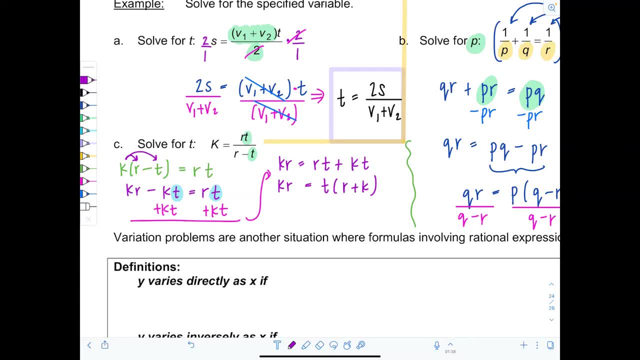 able to factor it out, And then dividing both sides by R plus K will finish off the job and T will be all by itself. So T equals KR divided by R plus K, And we are done All right, Good. So that's how to work with certain formulas that involve rational expressions. 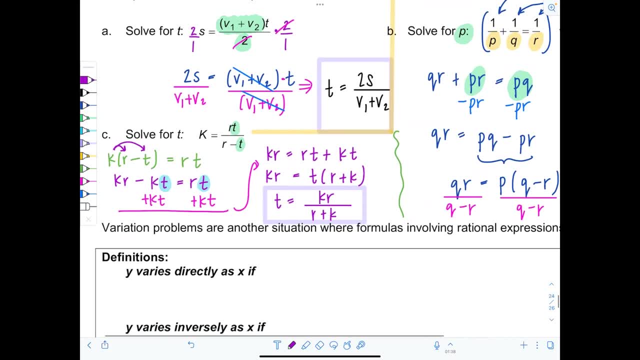 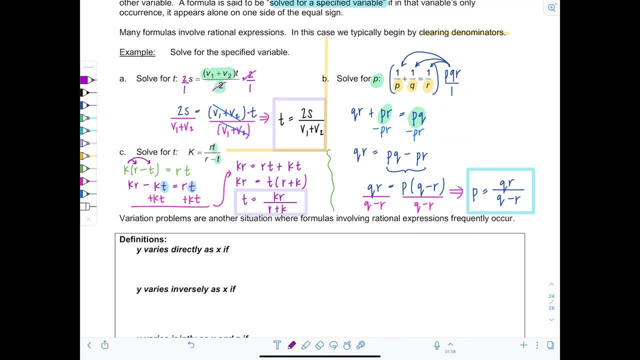 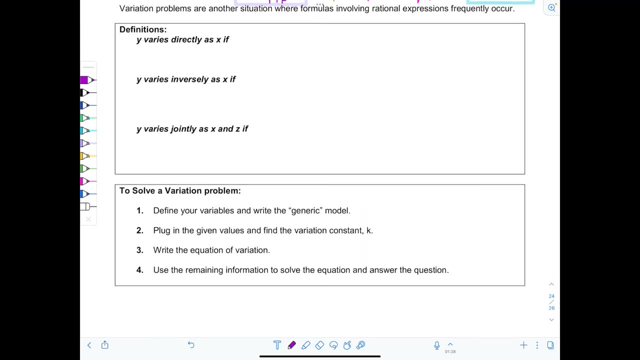 and isolate variables. Now, variation problems are another situation where formulas involving rational expressions frequently occur. So there's a little bit of terminology you have to get under control in order to solve these problems. We say that Y. variation problems are another situation where formulas involving rational expressions frequently occur.